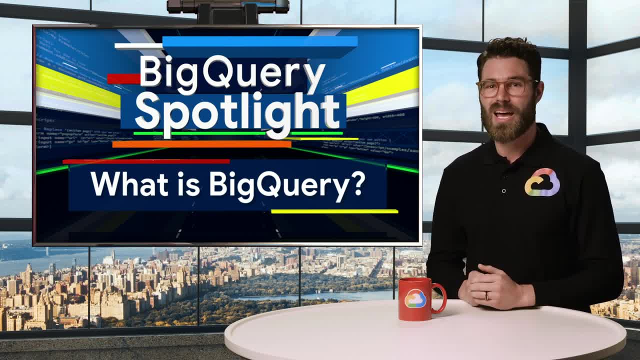 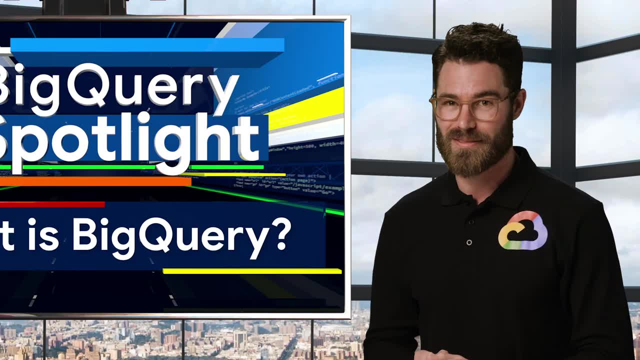 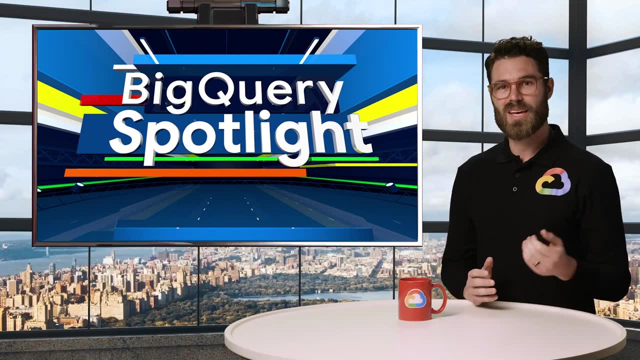 accessible to everyone. In this series, we'll show you how BigQuery can help you get valuable insights from your data with ease. Ask questions and get answers on BigQuery Spotlight. If you're a developer, data analyst or just about anyone else, you're probably working with data. 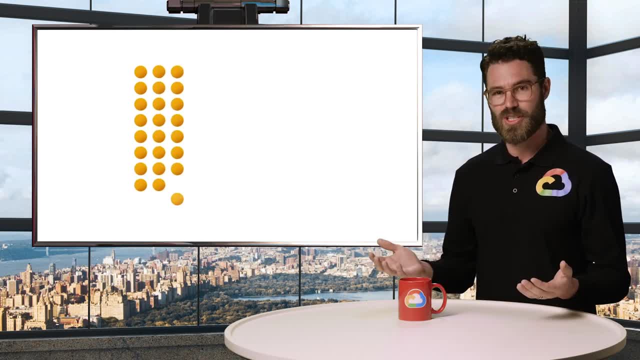 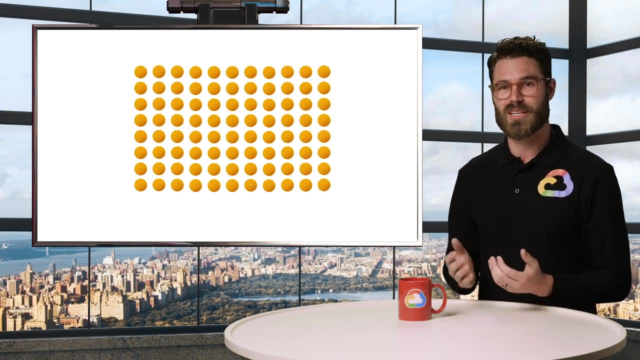 If your business has small amounts of data, you might be able to store it in a spreadsheet, But as your amount of data grows to gigabytes, terabytes or even petabytes, you start to need a more efficient system like a data warehouse. That's because all that data isn't very useful unless you have a way to analyze it. Traditionally, larger sets of data means longer times between asking your questions and getting answers. Have you ever needed to wait hours or days for an analytics report to be run? 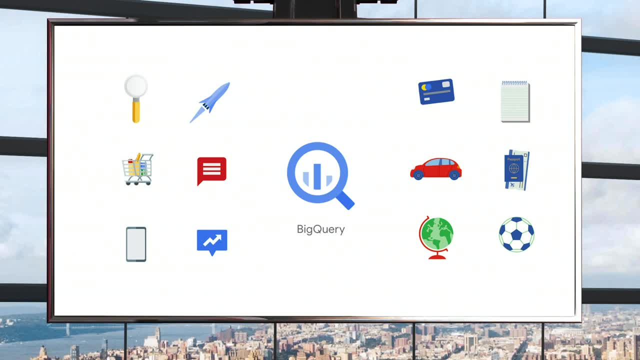 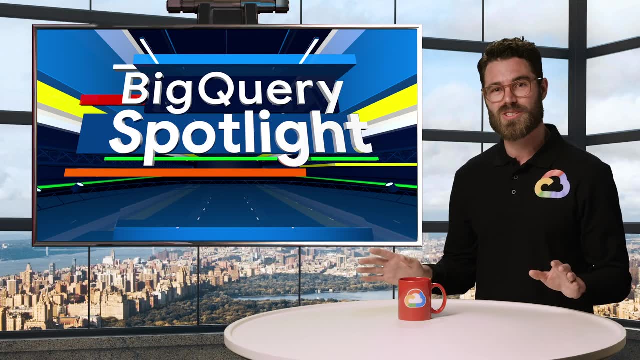 BigQuery was designed to handle massive amounts of data, such as log data from thousands of retail systems or IoT data from millions of vehicle sensors across the globe. It's a fully managed and serverless data warehouse, which empowers you to focus on analytics instead. 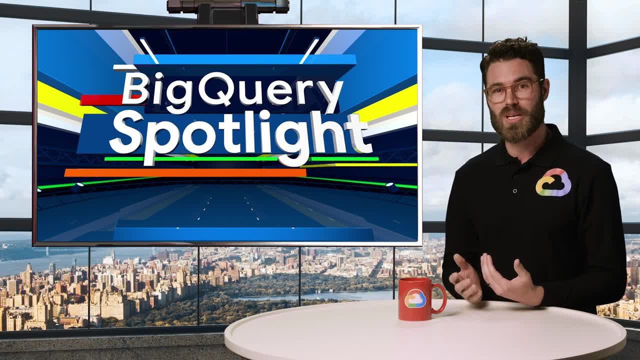 of managing infrastructure By design. BigQuery helps you avoid the data silo problem which happens when you have individual teams in your company having their own independent data marts. This can create significant friction between analyzing data across teams and cause challenges with data version control. 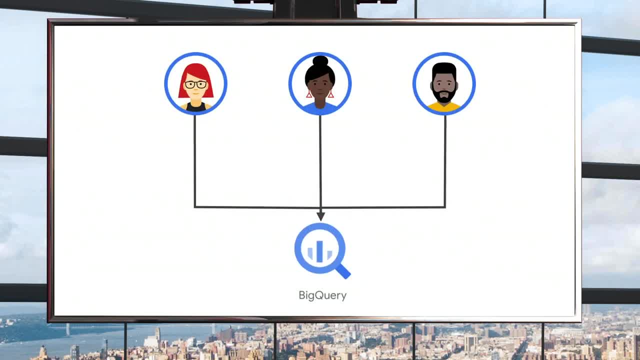 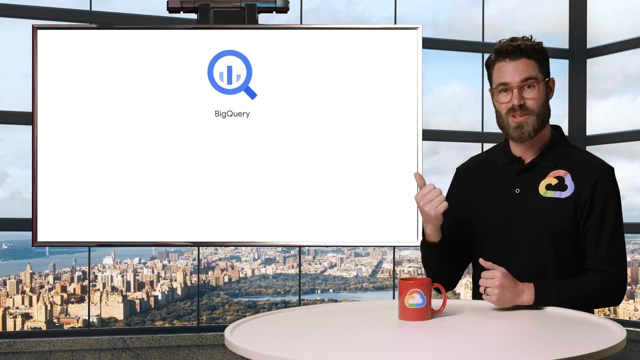 Thanks to the integration with Google Cloud's native identity and access management, you can assign, read or write permissions to specific users, groups or projects and keep your sensitive data secure, all while still collaborating across teams. Working with data in BigQuery involves three primary parts. 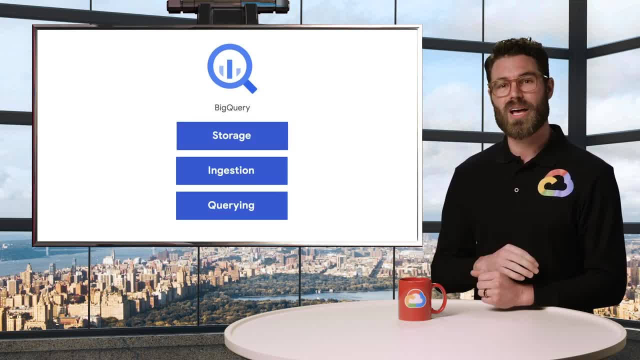 storage, ingestion and querying. Google handles running everything else. BigQuery is a fully managed service, which means you don't need to set up or install anything and you don't require a database administrator. You can simply log into your Google Cloud project. 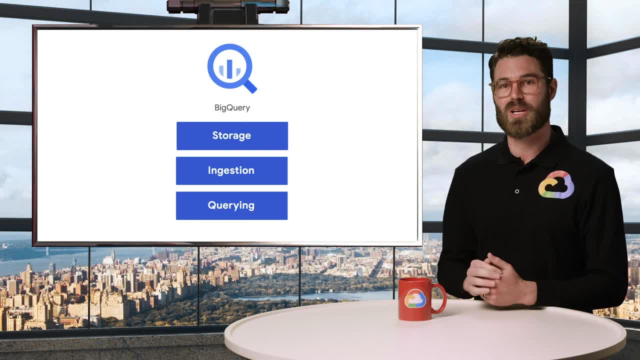 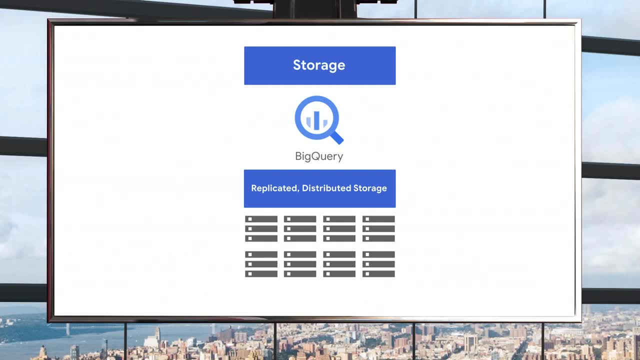 from a browser and get started. First, let's talk about BigQuery storage. Data is stored in a structured table, which means that you can use standard SQL for easy querying and data analysis. For example, let's say that you have some data that represents the sales for each of your stores. 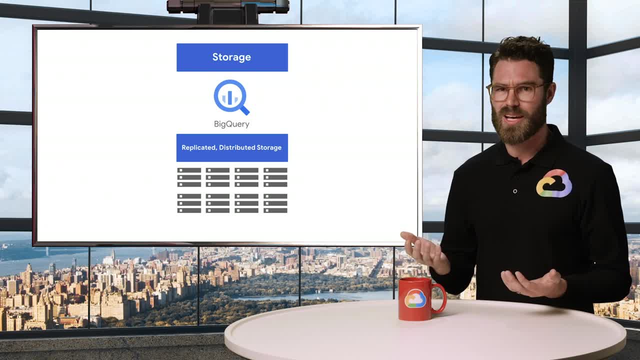 in the last year. You could probably use a smaller database for that, but what if you have thousands of stores? And what if you want revenue broken up by product skew or by region per time period? BigQuery is perfect for big data because we